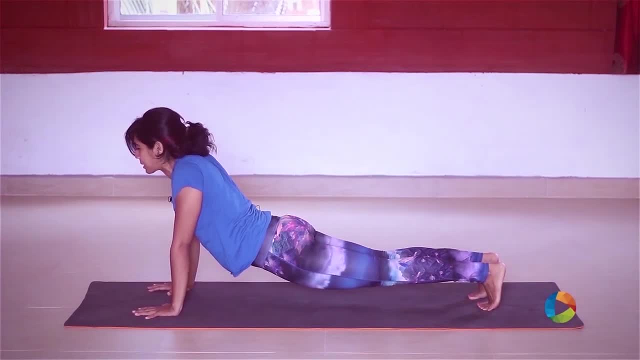 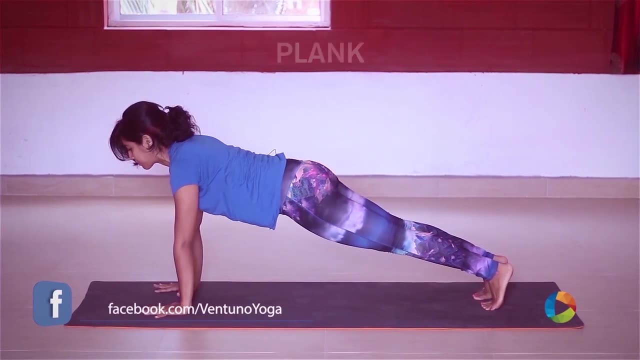 tendency to do this or drop your hips. That's really bad because you'll hurt your lower back. So always pull through your belly and make sure the body's in a straight line, Roll the shoulders and keep the body really nice and long and engage your thigh muscles. 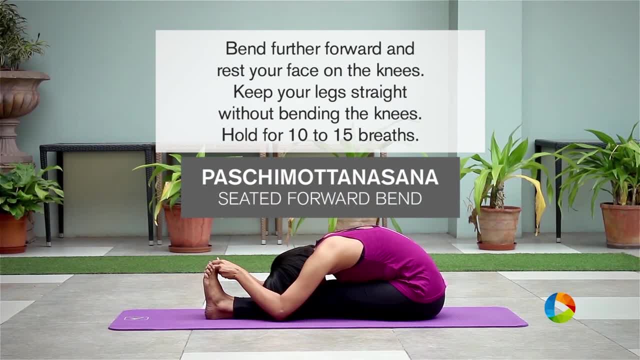 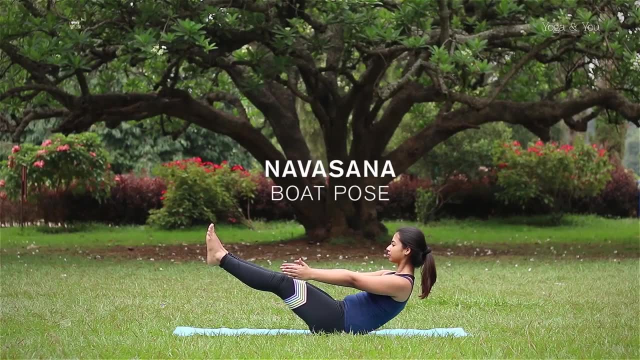 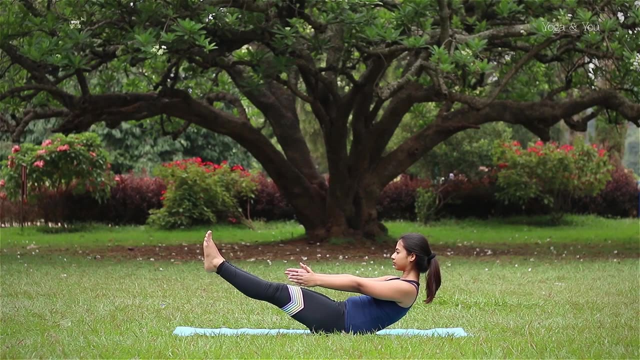 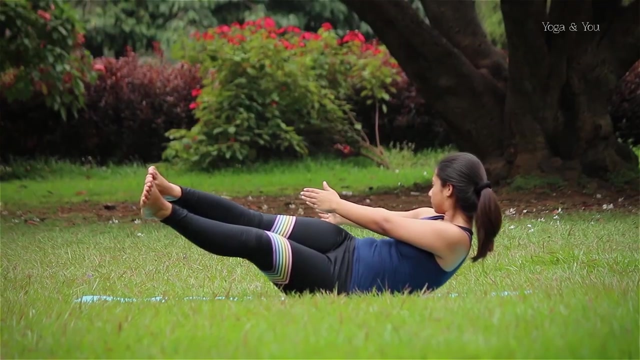 In Naukasana, making sure that our core is engaged, our knees are straight and holding it for a minute, Followed by Kati Naukasana. You can either put your hands up or elbows down for 30 seconds on each side. 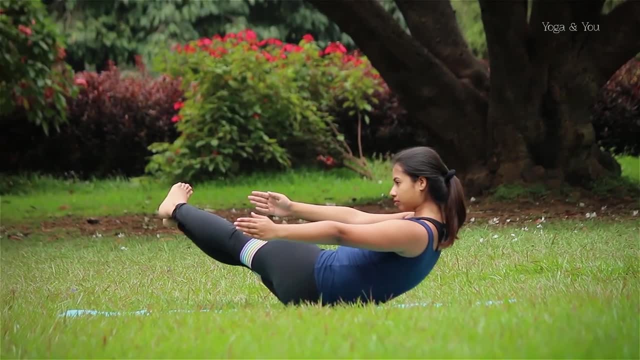 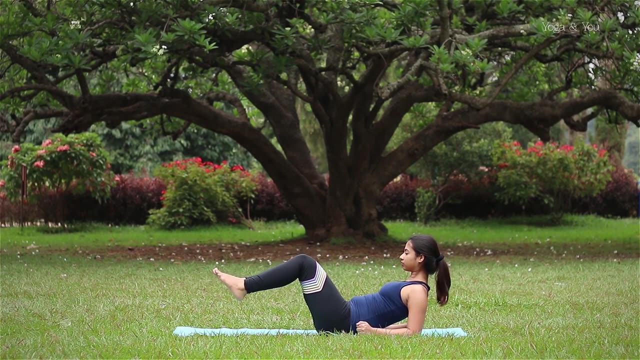 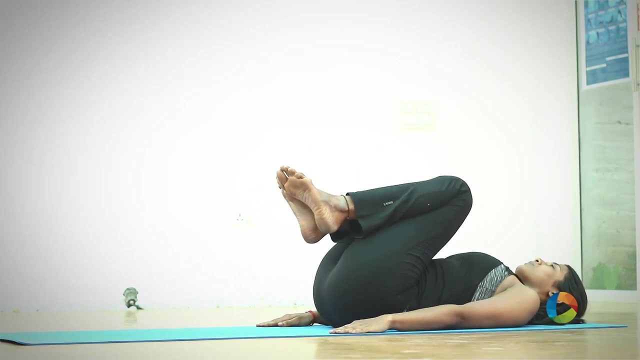 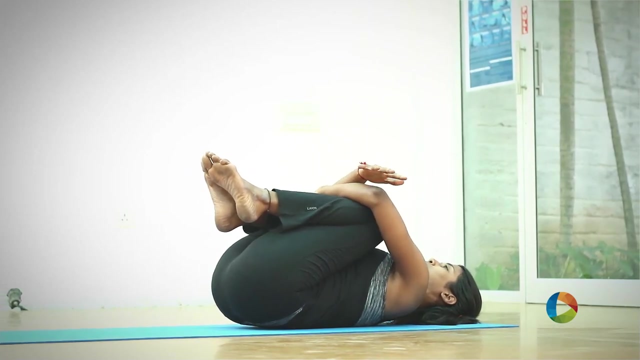 The rest posture, Engaging our core again and holding it for another minute. Now gently take both the knees towards the chest. Interlock your hands. If you want more squeezing of your right leg, you can do that. You can hold both the sides of your elbow. Pull the navel inside as you exhale. Try taking. 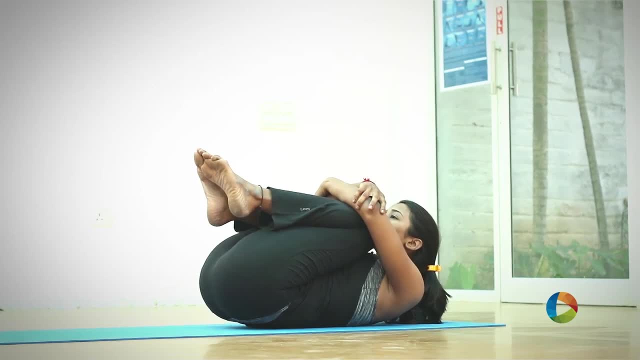 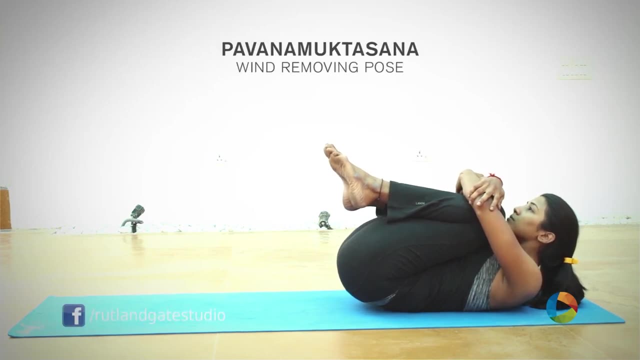 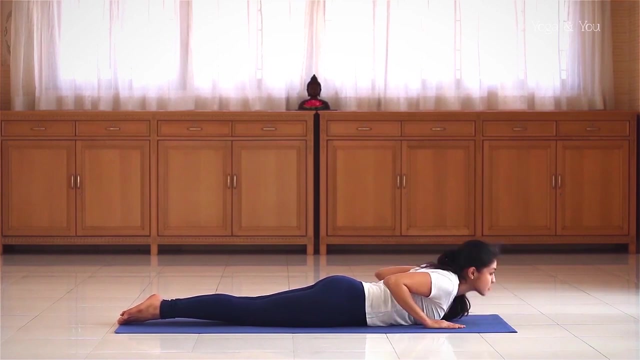 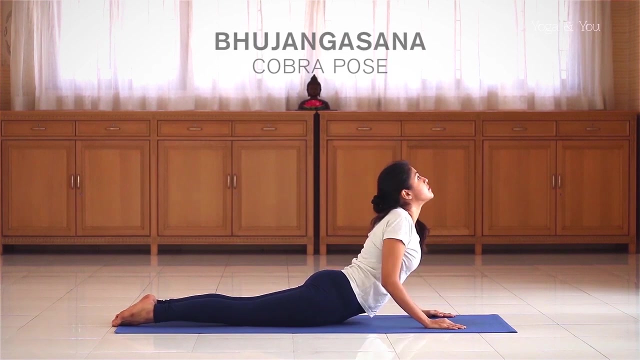 the chin towards the knee. Don't take your forehead to the knee, Then you'll be hurting your neck. Move the palms just beneath the shoulders. Inhale head up. Elbows straight Feet together. Exhale head down. 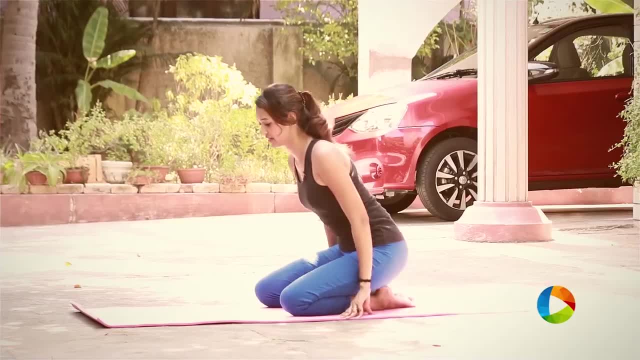 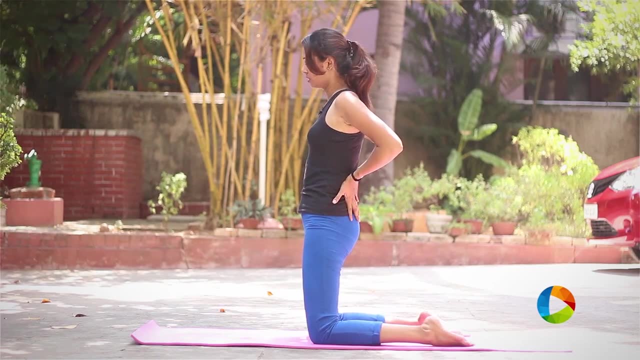 So begin by sitting in Vajrasana And what you want to do is basically stand onto your knees and widen your legs- really nice. Bring your palms facing down, your fingers facing down onto the back of your hip and slowly inhale first and exhale slowly, Push your. 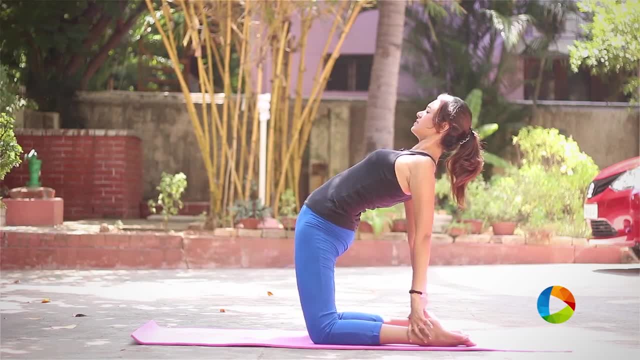 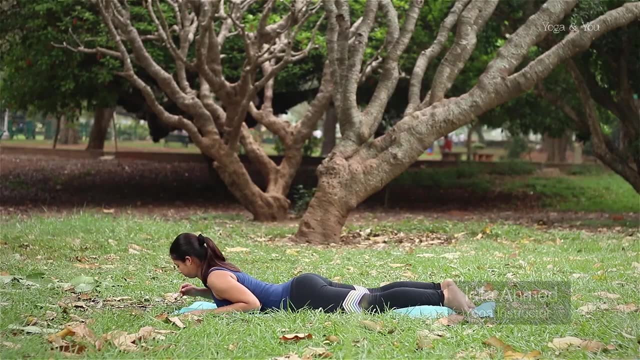 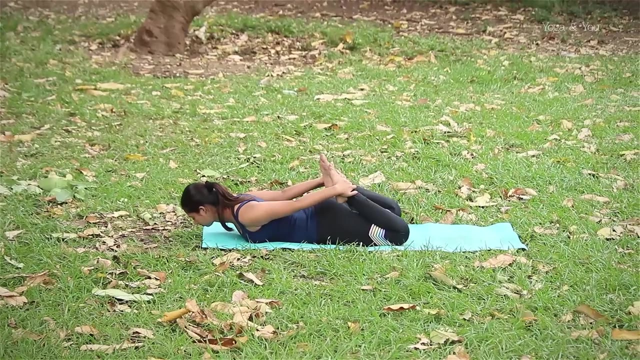 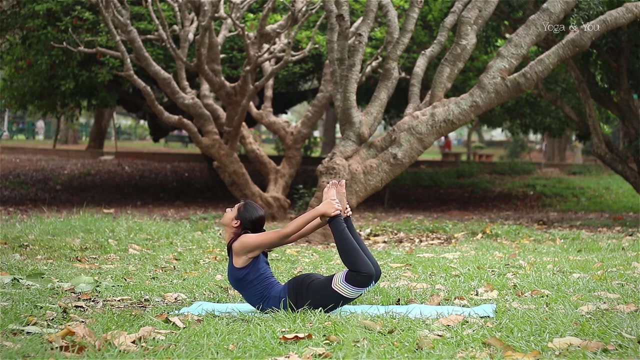 hips forward and slowly bringing your arms to your ankles And arch back. So to perform this asana, lie down on your stomach, Hold both your ankles And start to pull your ankles and lift your body up. If you look up, it'll help you go even higher.